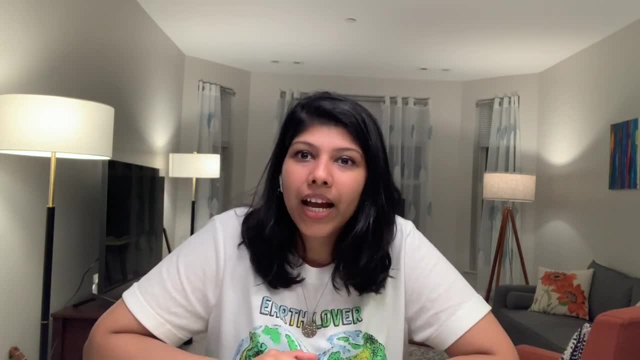 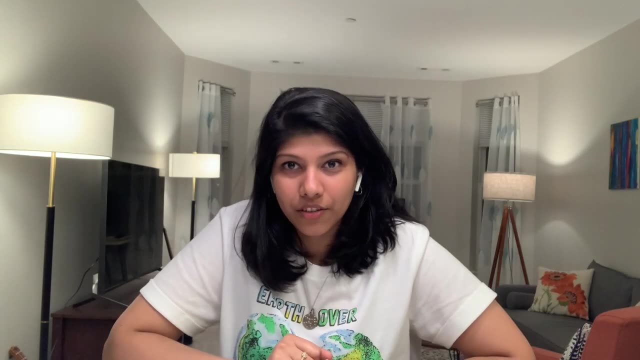 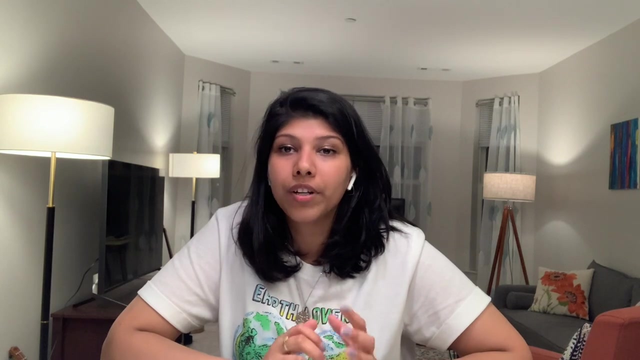 background. Second would be the course I took at Northeastern and third would be about the living experience in USA. So let's begin with addressing the first question about profile and background. So I had about three years of work experience in India, which was inclusive of an Android. 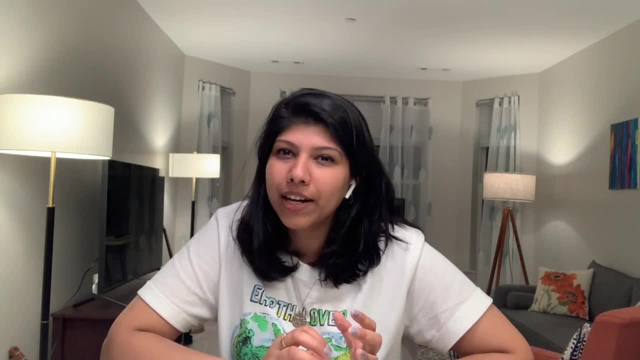 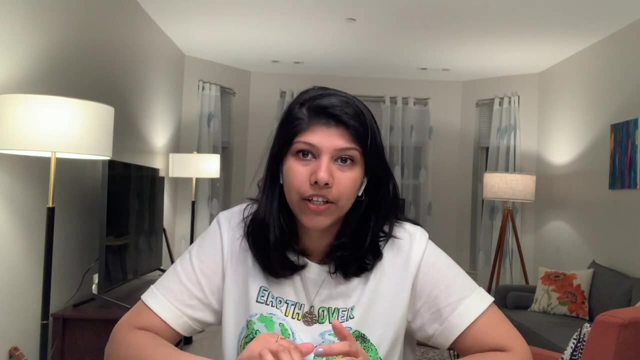 development profile as well as a BA profile. So initially I was into Android development, but I took a great switch and moved into associate analyst and business analyst role, which was more into SQL, Hive Table, Dash, coding and that's how I got interested in data. 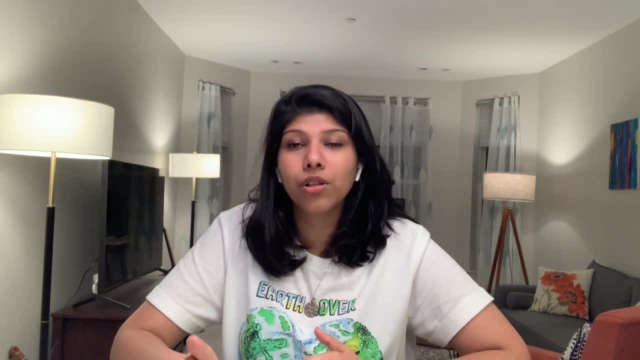 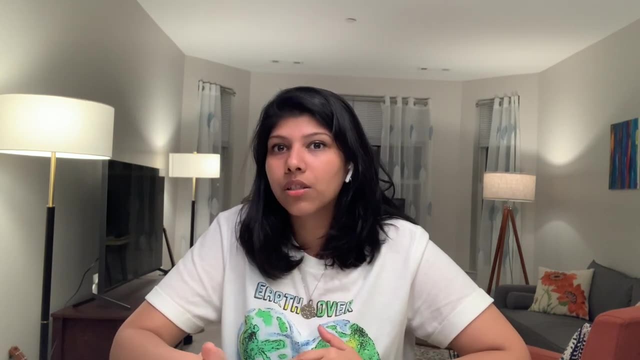 And then I was looking into courses which were more aligned with data and also had some similarities, which I wanted to do. going forward, In shortlisting all the courses, I found out that Northeastern's course was aligning quite well with what I really wanted to do, and hence I chose the course. 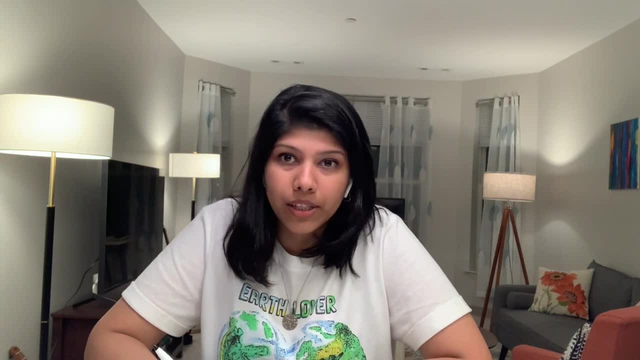 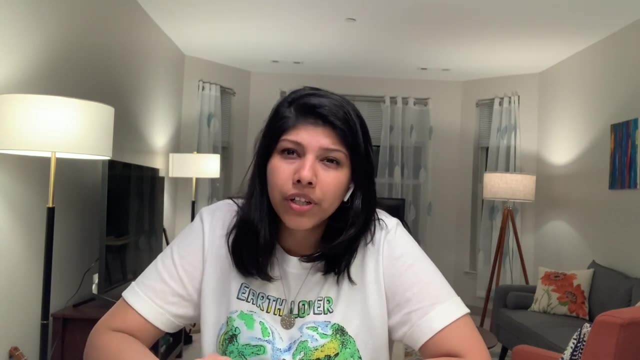 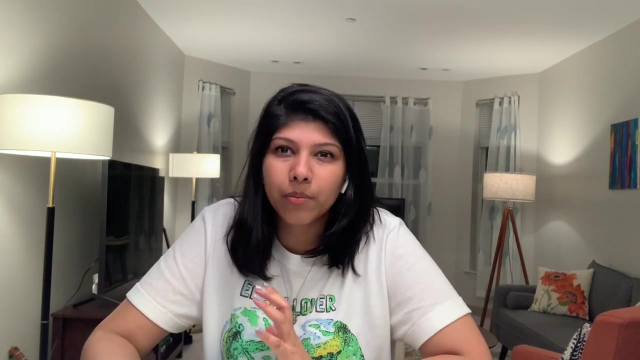 Coming down to the second question, So I would like to address the course that I did. I came to Boston Northeastern University and did a course of masters in professional studies in analytics, So there are three different courses of data at Northeastern. That's how the situation was when I came in 2017 fall. there might have been some additional. 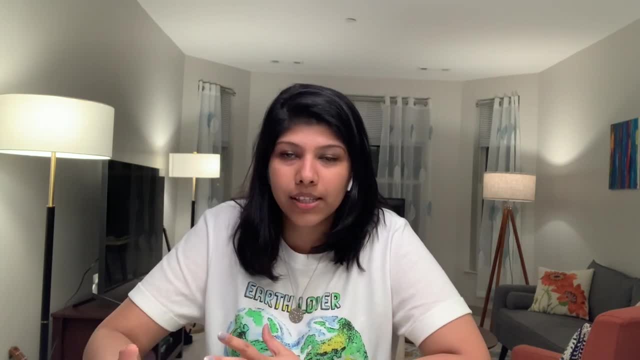 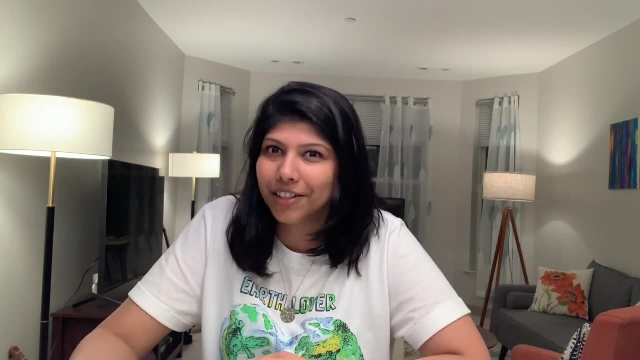 courses post that, but, as of my knowledge, these are the three courses that exist at Northeastern: One is a data science program in CCIS, The other is a COE program, which is of data analytics, And the third one is a master's in professional studies- analytics- CPS. 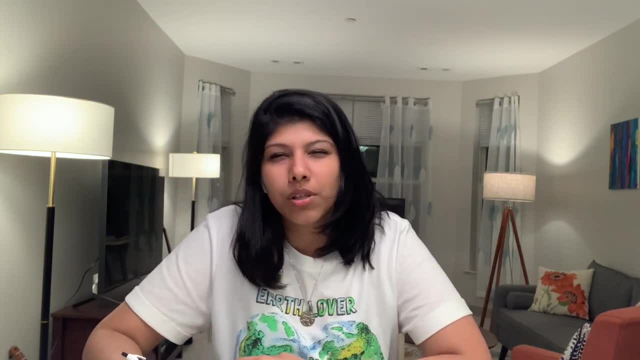 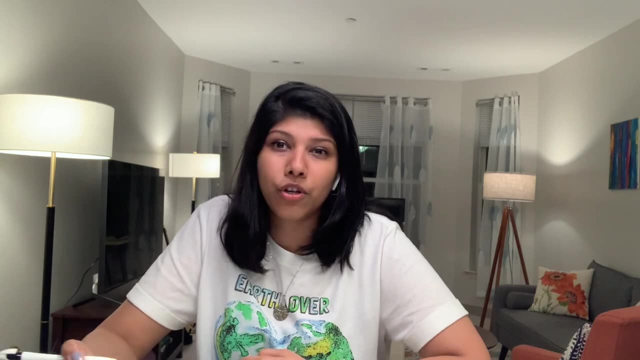 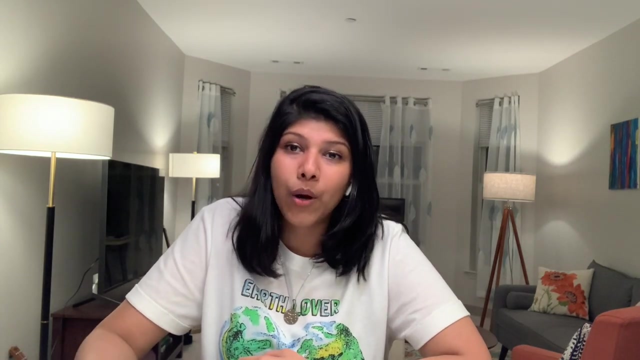 which is what I chose to pursue. So this course was interesting to me because it had various pillars of the strong data science, data analytics or engineering profile that you want to build going forward. To begin with they have five, four core courses and then you have three different. 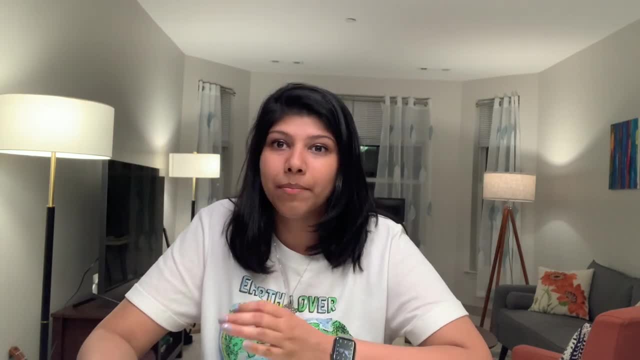 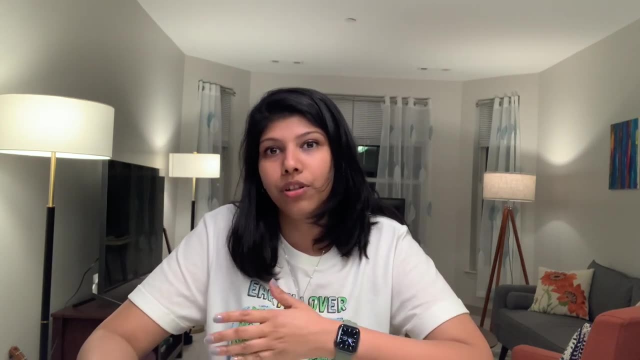 concentrations and you can choose one concentration out of those three, depending on, again, what you really want to do going forward. Then you have some electives and then there is a capstone and experiential learning program. So the courses well balance and divide into various structures. 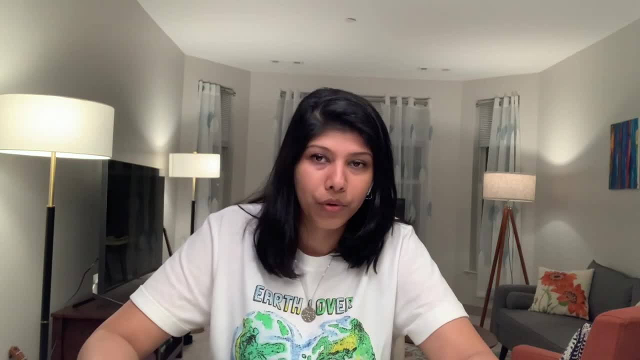 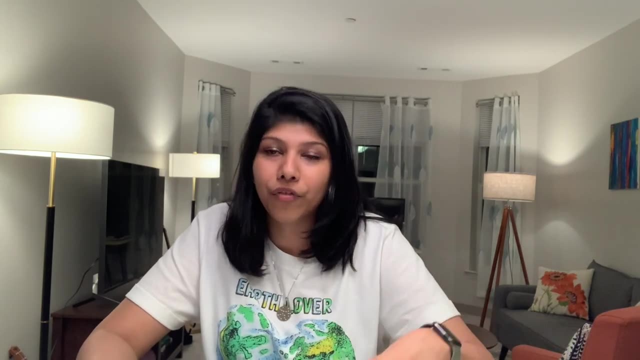 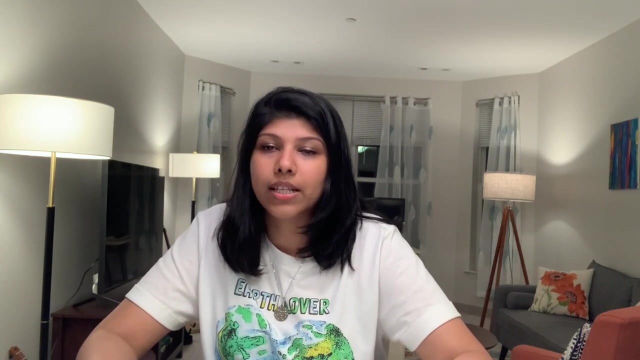 and you can choose your path going forward while you are into this program. Just to keep it brief, in this video I'll talk about the three different profiles and concentrations that you can build on. There is statistical modeling, the other one is applied machine intelligence and the third one 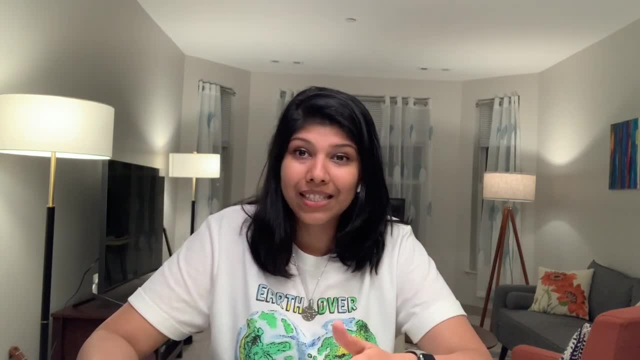 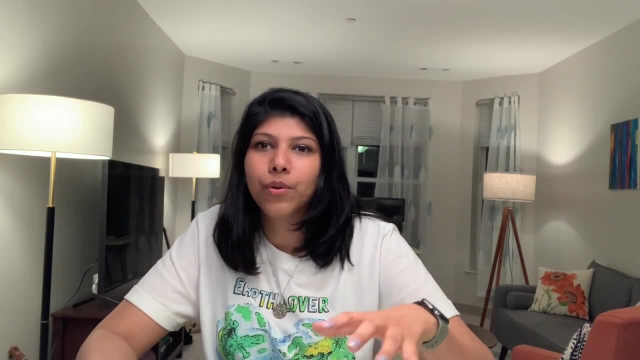 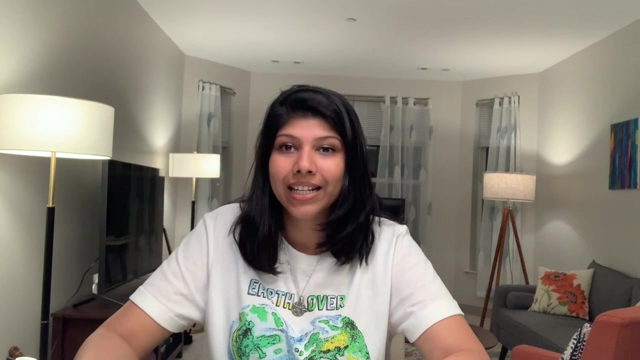 is evidence-based management. So when I came in 2017, the second one, which is applied machine intelligence, wasn't really a core concentration, but it was built over the time. But I was lucky enough to choose my electives From this four points of concentration, although my concentration was statistical modeling, and then 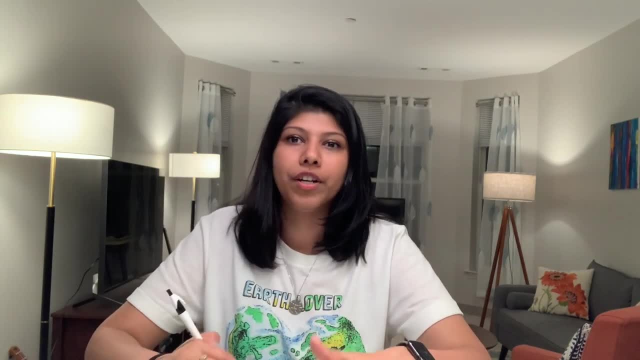 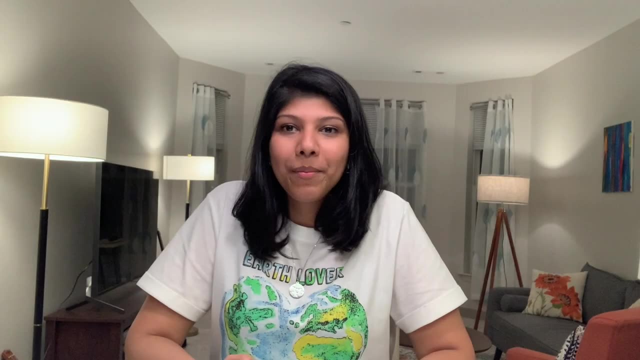 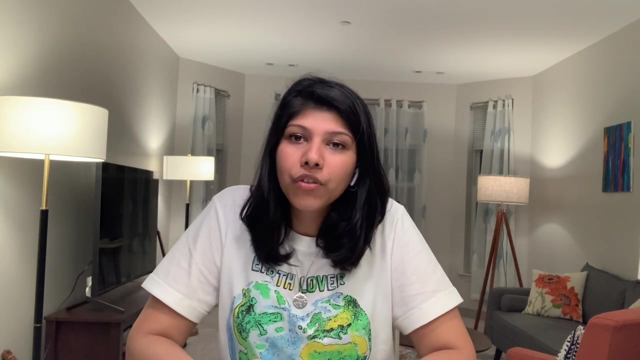 I chose some electives from artificial intelligence, so I had a mixed profile of a data scientist as well as a data engineer. So, coming on to the next question: life in US. So right now I'm working as a data scientist at a Boston tech company, For most of the time in US. I've been in Boston for about two and a half years. 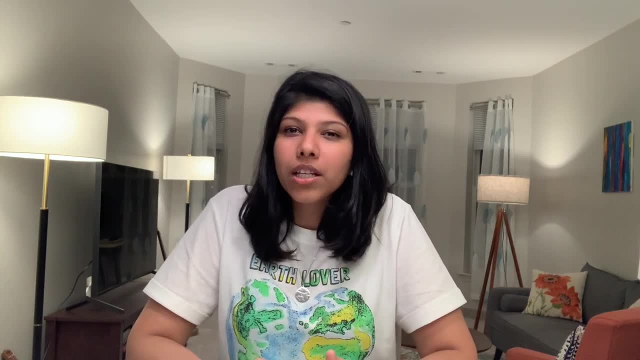 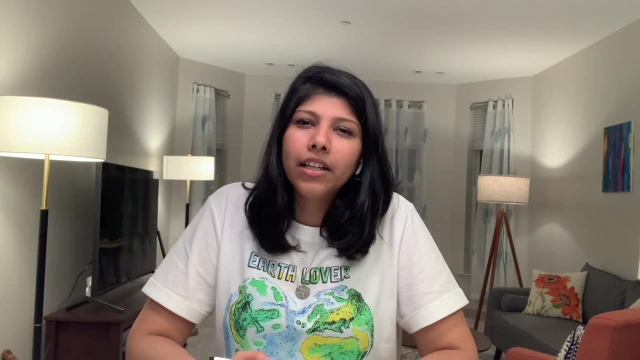 and six months in Michigan for my co-op. Let's get started. So working is key, is really important for you to develop a career that you really want for yourself. There are a lot of tech events that keep happening around the city where you can go. you can sign up. 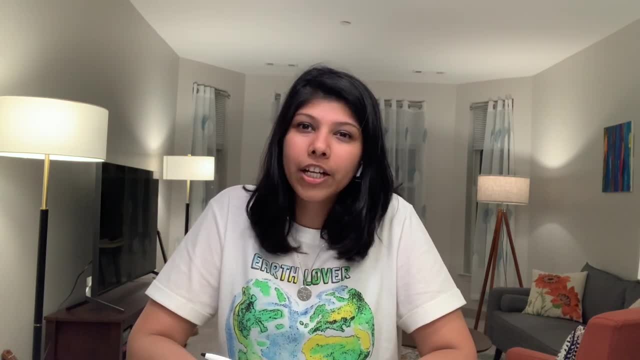 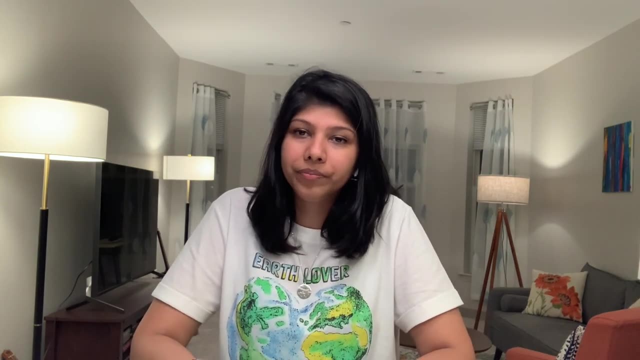 for free, attend those events and gain a lot from them. It kind of gives you an insight as to what's really happening around the tech companies and what kind of job opportunities are really available. The next is there are various tech talks that keep happening on campus. 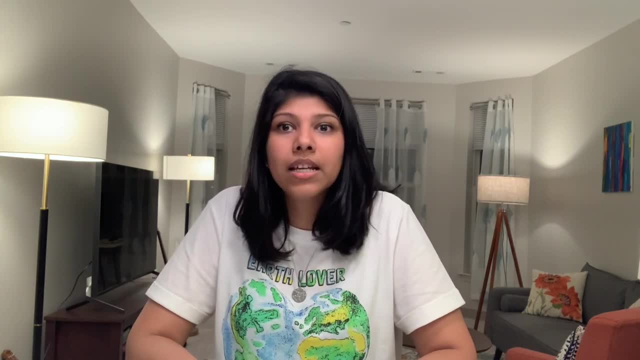 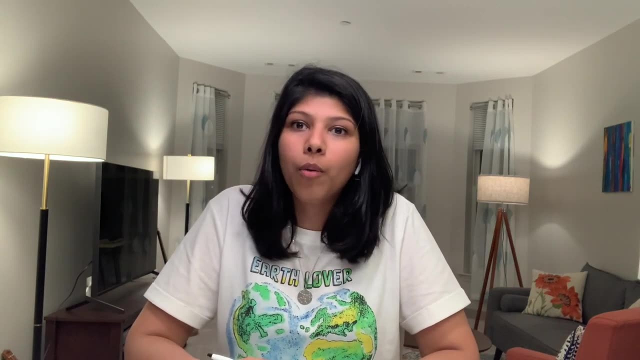 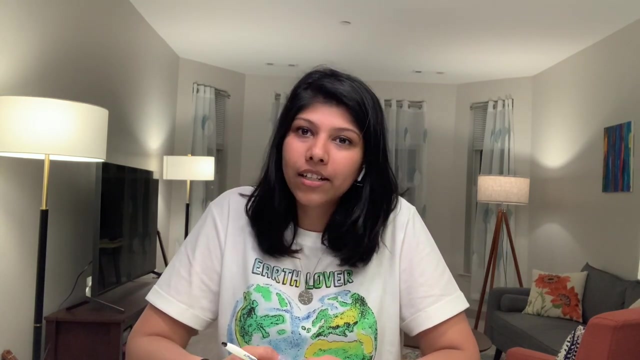 Professions from big as well as small companies come to campus, give a walkthrough of what projects they're working on, what skill sets are required and also what job opportunities are available in their company. You can always connect with them via LinkedIn once the event is over and get in touch with them as necessary. 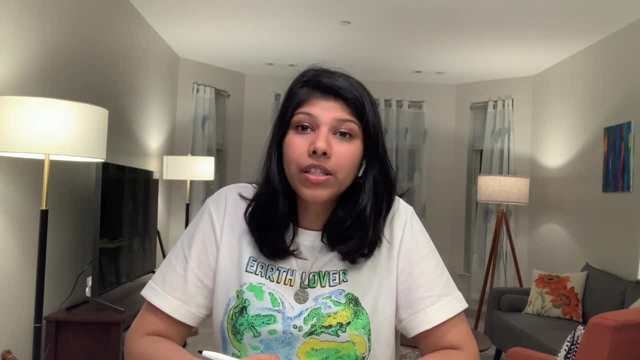 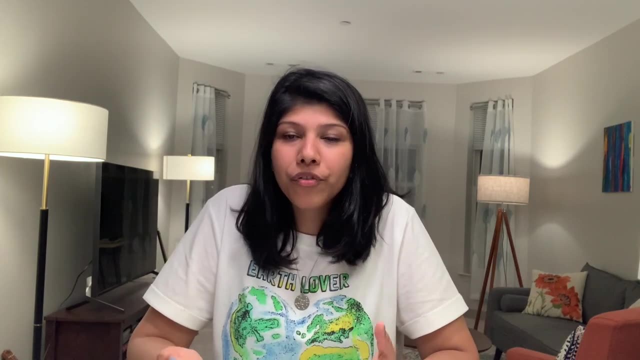 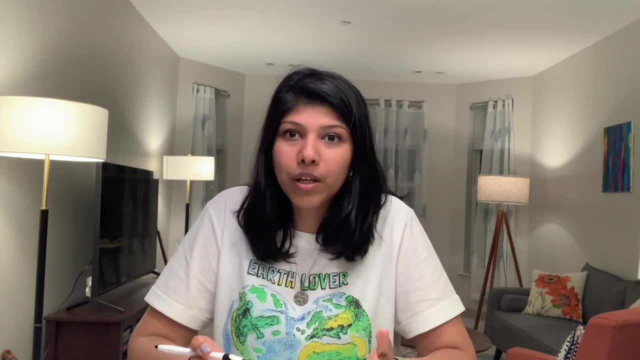 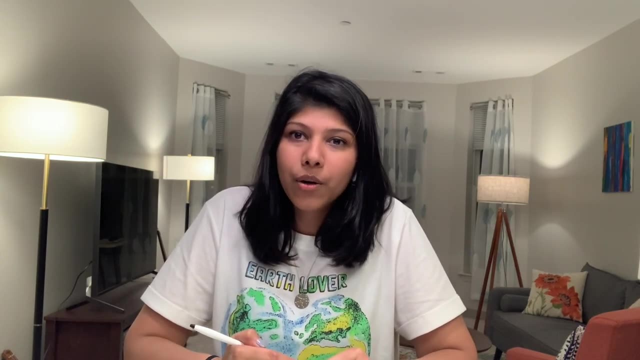 They can help you shape your resume so that it's more industry fit. Moving on to the next point, Northeastern offers seasonal career fair where companies- again big and small, and also medium-sized companies- come in to hire professionals for a fresh career and also for.